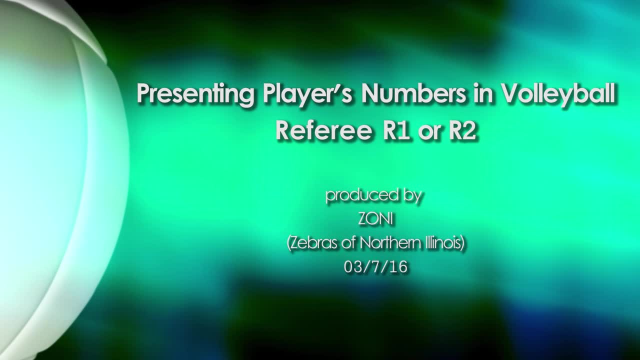 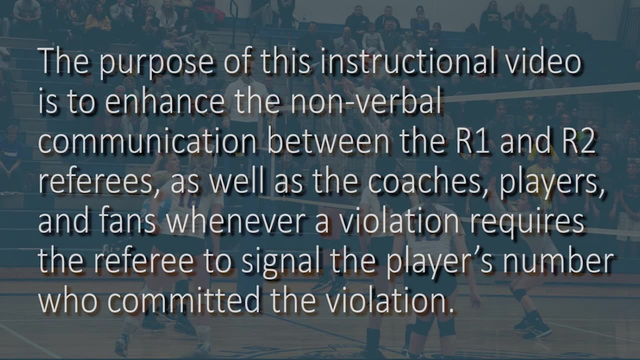 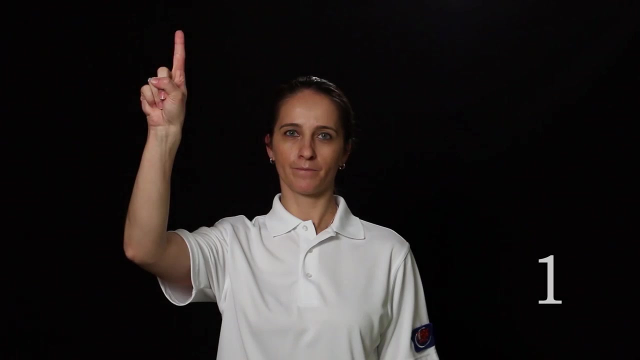 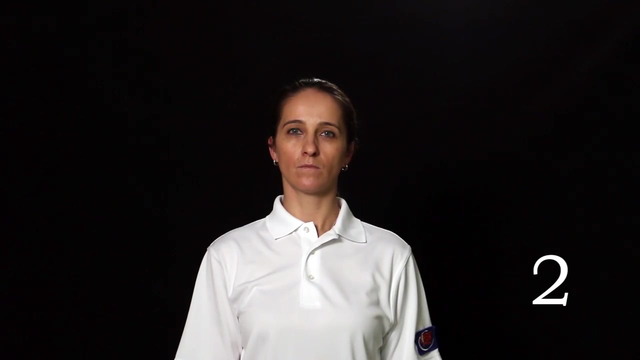 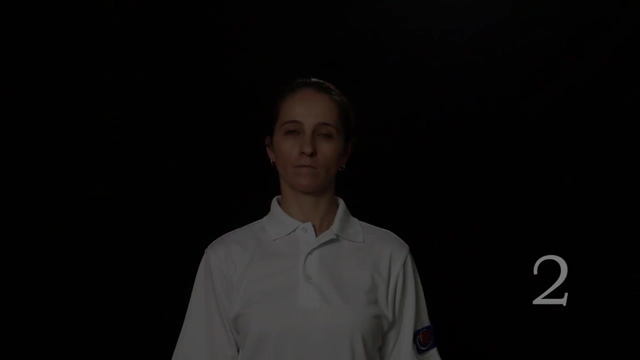 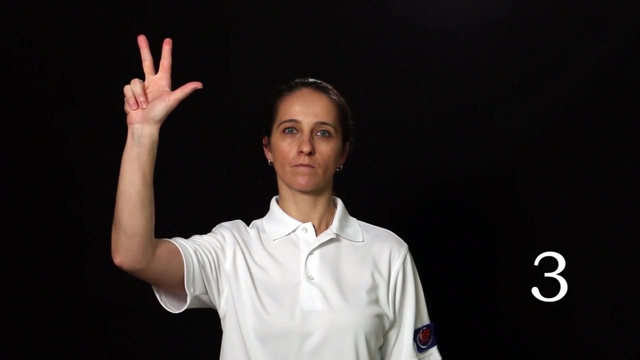 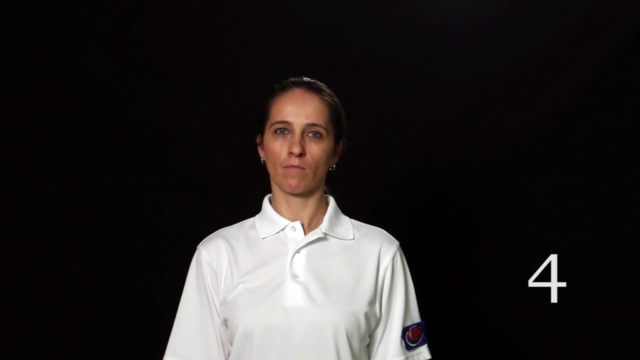 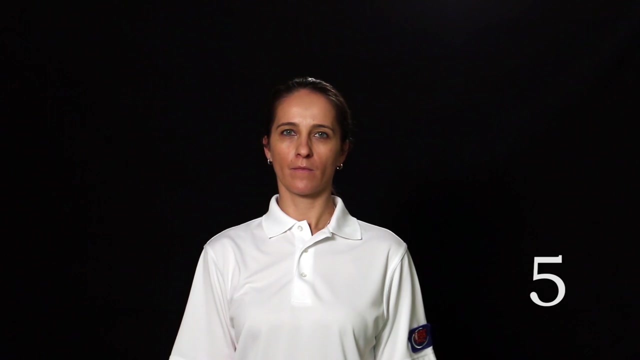 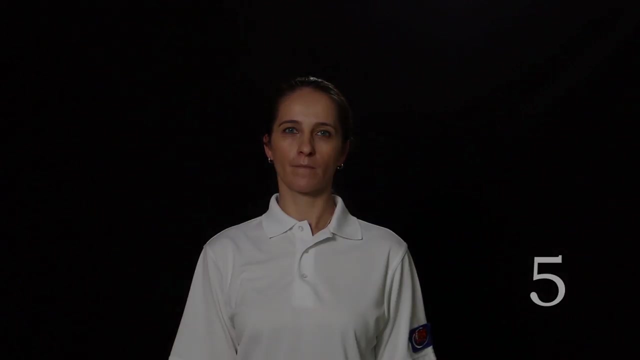 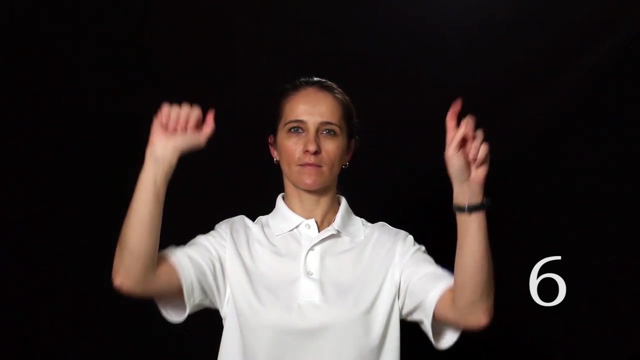 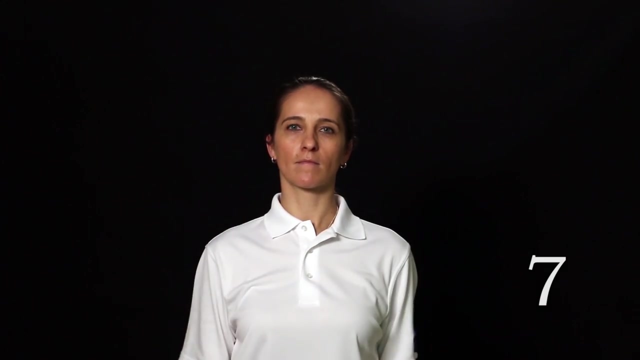 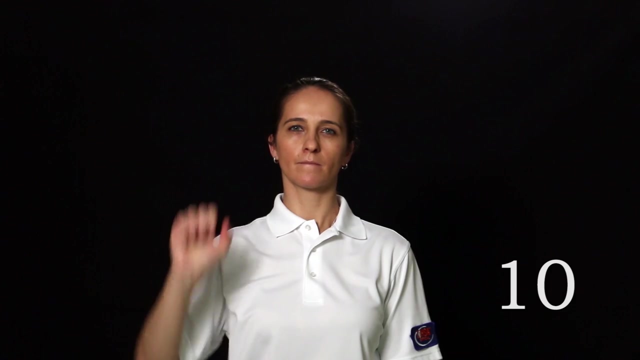 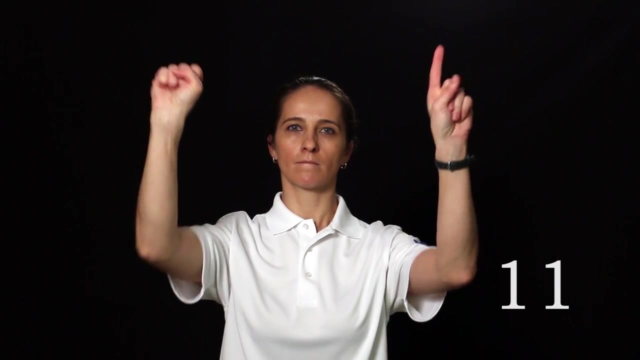 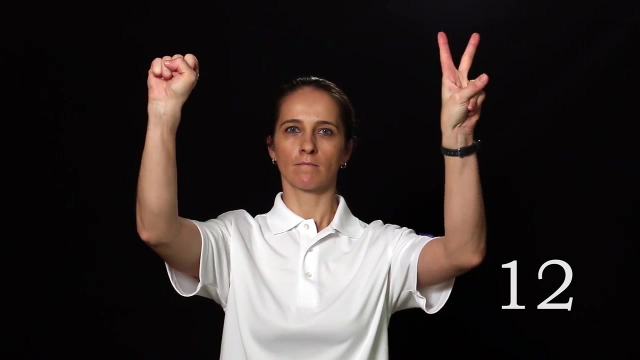 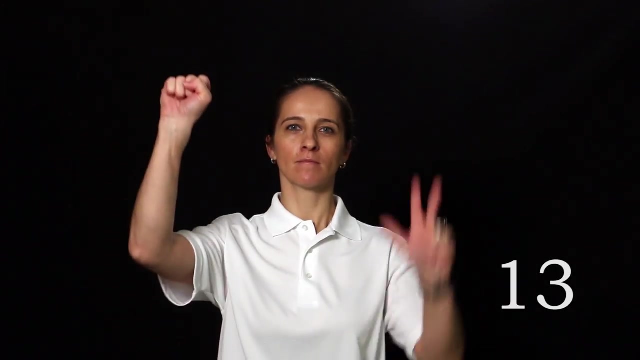 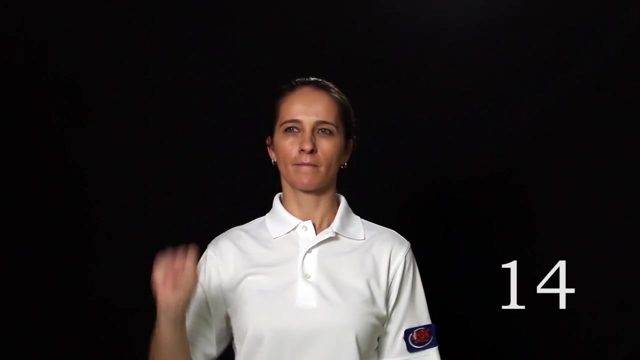 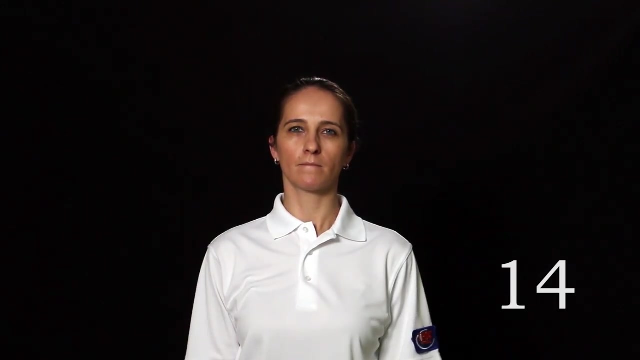 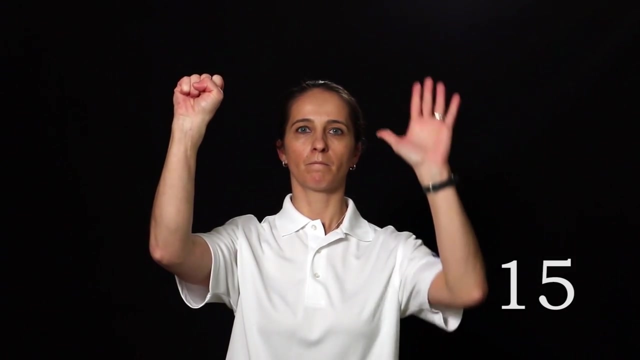 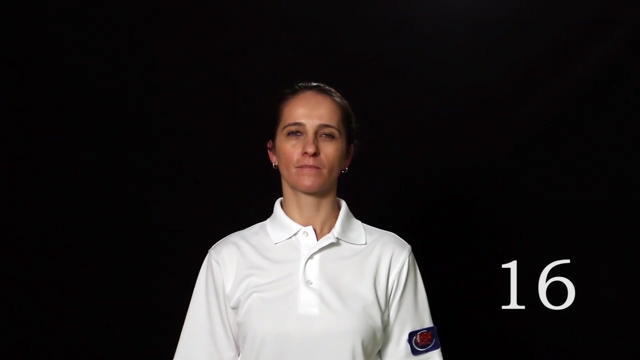 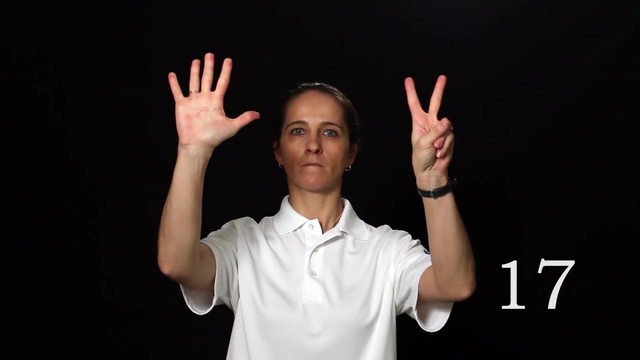 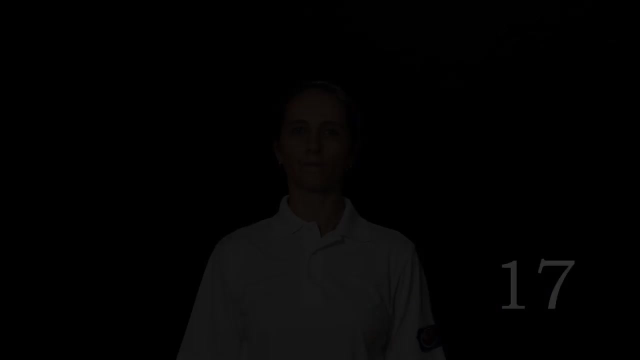 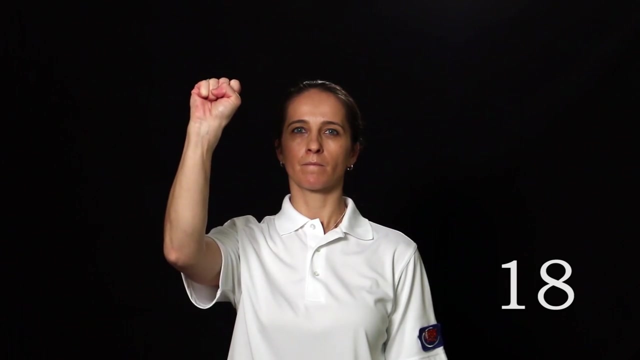 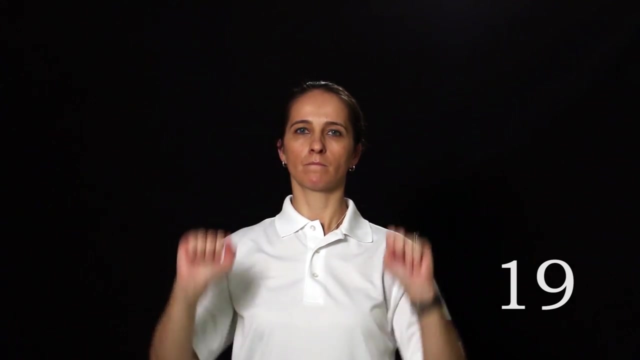 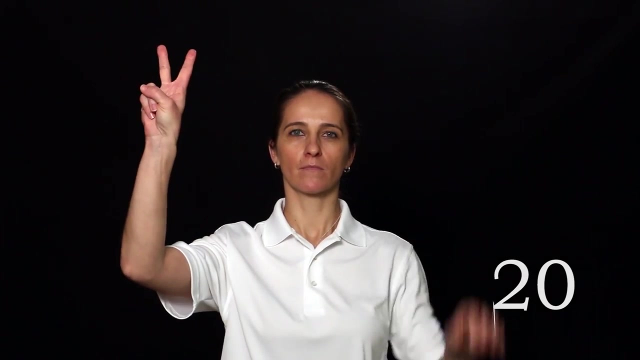 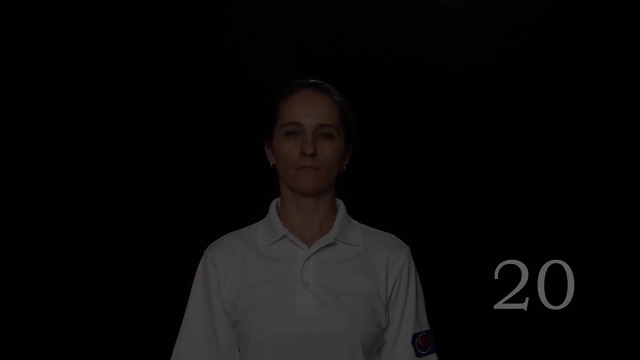 One, Two, Three, Four, Five, Six, Seven, Eight, Nine, Ten, Eleven, Twelve, Thirteen, Fourteen, Thirteen, Fourteen, Fifteen, Sixteen, Seventeen, Eighteen, Nineteen, Twenty, Twenty-one. Twenty-one, Thirty, Thirty, Thirty-two, Forty, Forty-three, Forty-three, Fifty, Fifty-four, Fifty-four, Fifty-four, Sixty, Sixty, Sixty-one, Sixty-six, Seventy, Seventy, Seventy-two, Seventy-seven, Seventy-seven, Eighty, Eighty, Eighty-three, Eighty-three.